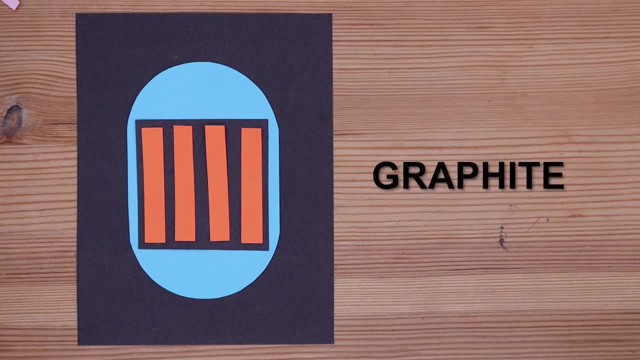 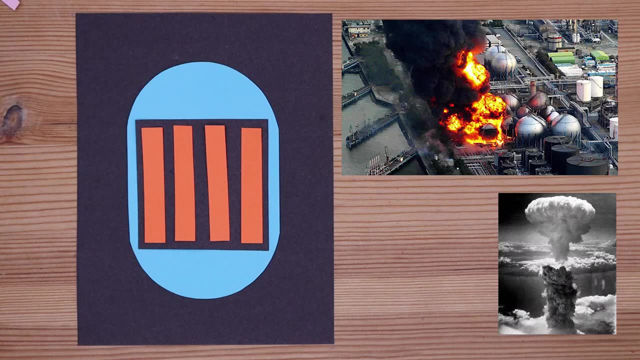 that they can easily be absorbed. We can use graphite as a moderator. What if there are too many chain reactions going on? Too much fission can lead to overheating of the reactor. When the rate of reaction is too high, we need to lower control. 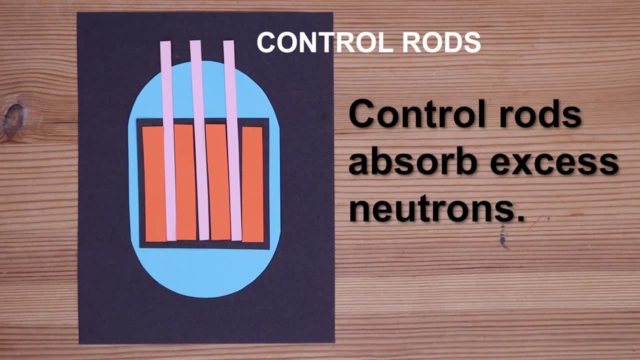 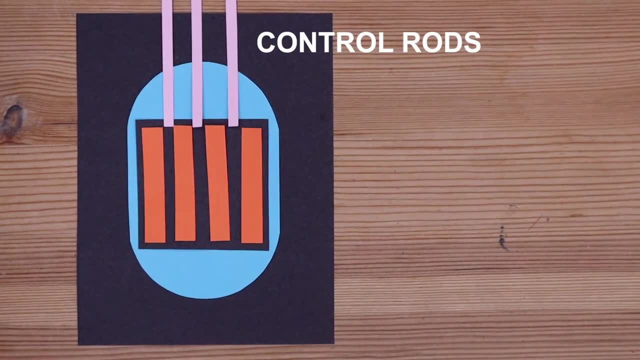 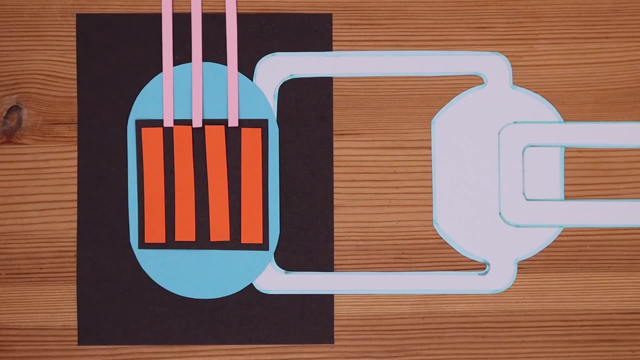 rods to absorb neutrons, preventing them from traveling between fuel rods. Once these reactions are reduced to a safe rate, we can then raise the control rods. A typical nuclear reactor functions at 300 degrees Celsius. That's a lot of thermal energy. You want to pump coolant, which could be water, into the reactor to absorb. 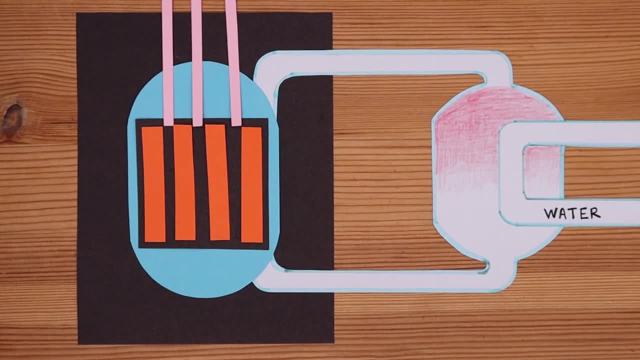 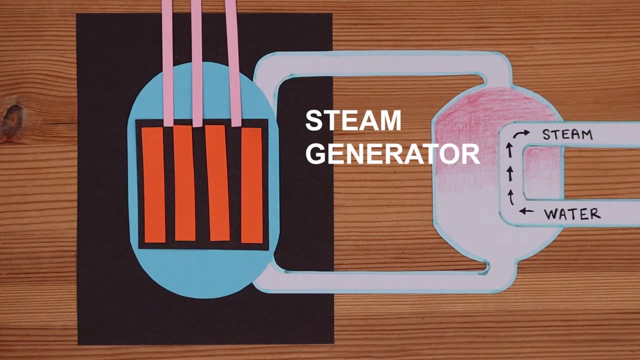 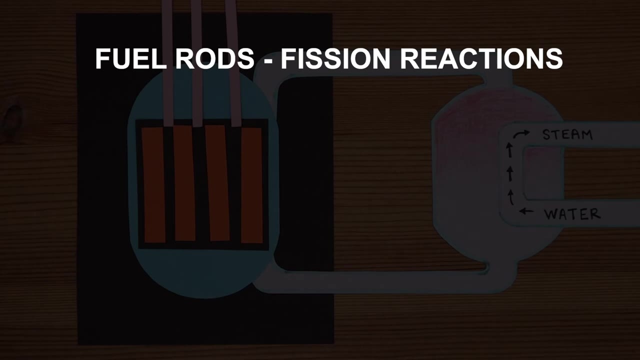 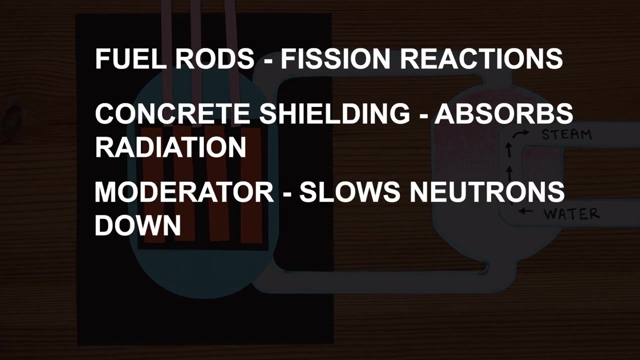 and transmit the energy out of the reactor. If we pump water into the steam generator, the steam created can then drive a turbine. The turbine generates electricity. To summarize, fuel rods are where fission reactions take place. The concrete shielding prevents radiation from leaving the reactor. The moderator slows neutrons down so that 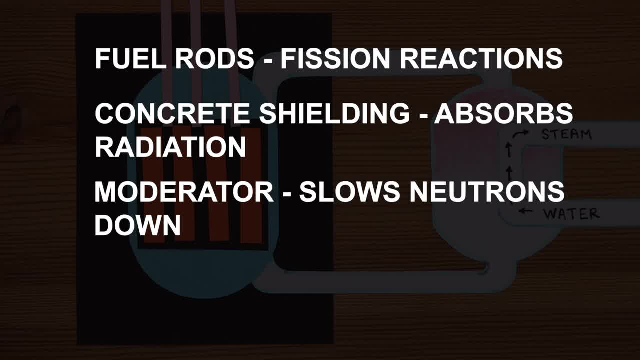 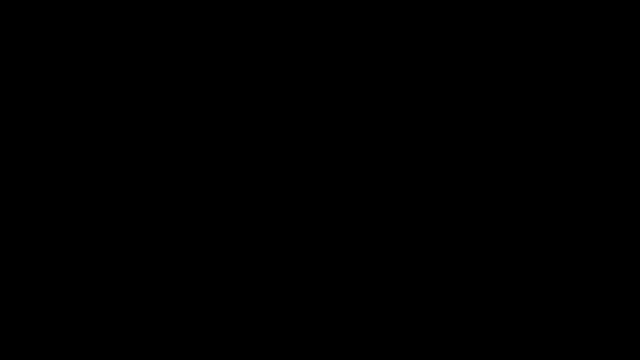 they can easily be absorbed by fuel rods. When the rate of reaction is too high, the control rods are lowered into the reactor to absorb excess neutrons. We'll see more of those in the coming episodes. 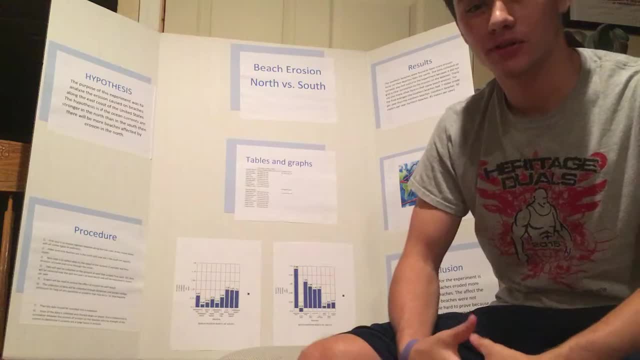 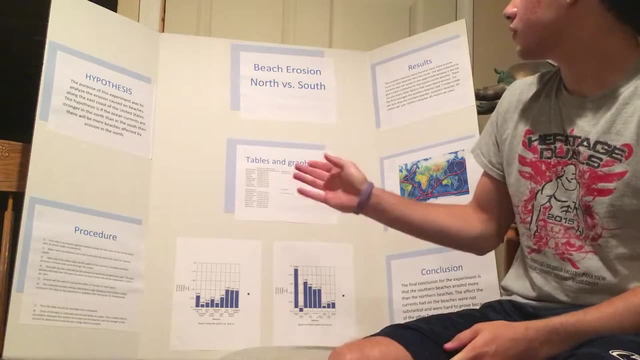 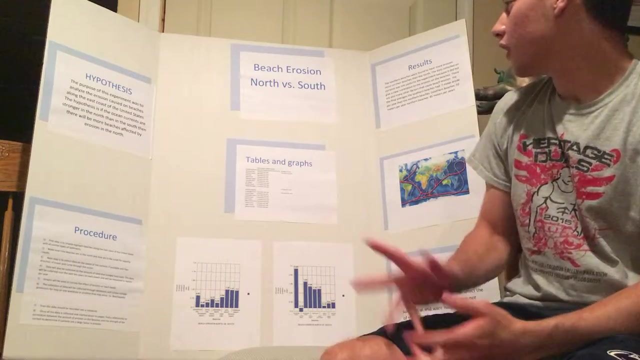 Hi, my name is Matt Oswald and this is my independent science research project. So what I did my project on was I chose to research beach erosion along the east coast of the United States and what I wanted to do was compare the north half of the east coast. 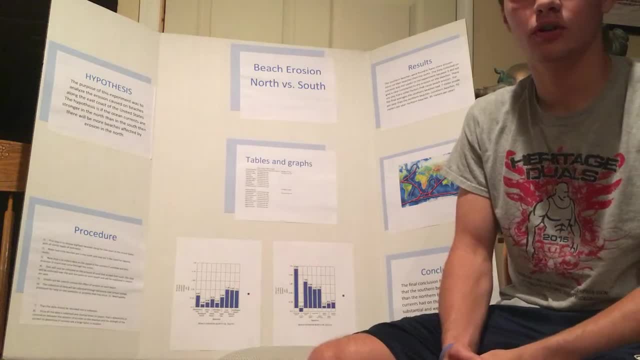 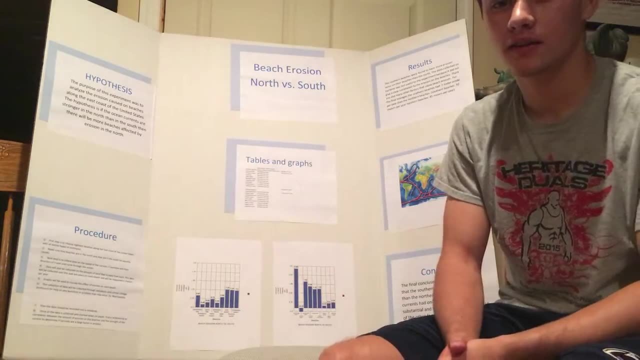 compared to the south half and also see if there is a correlation between currents and how much they affect erosion on those beaches. So for my hypothesis I said that the northern half of the east coast would erode more than the southern half, and I got this hypothesis from looking at 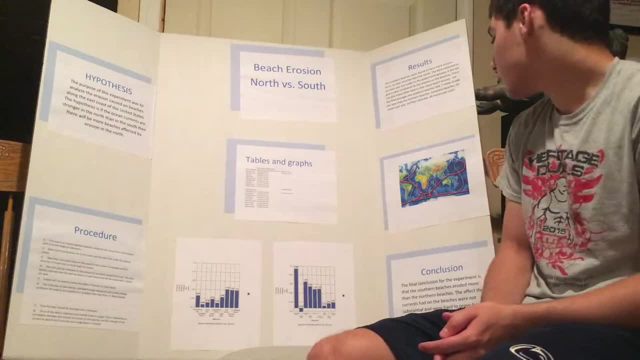 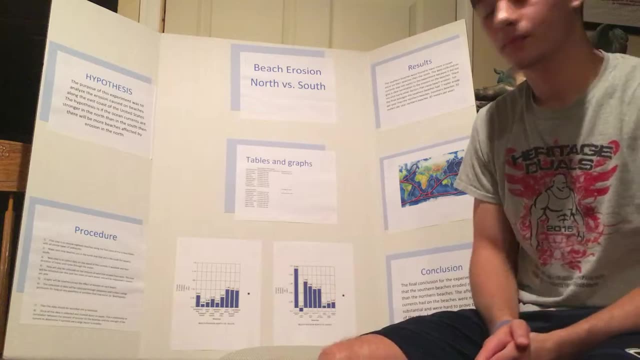 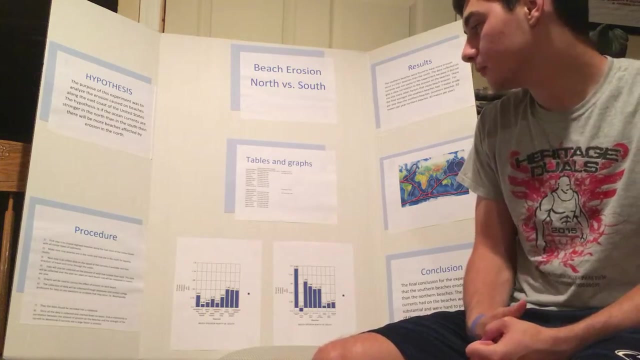 the Coriolis effect. and when you look at the Coriolis effect you can see that it is closer towards the northern half than it is towards the southern half where the gulf stream jets out away from the east coast. So for my procedure it was fairly simple. I picked 18.